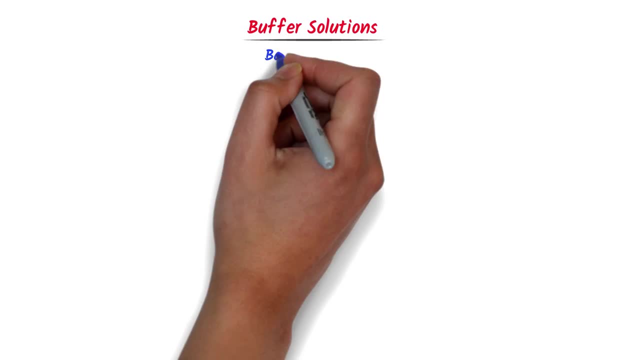 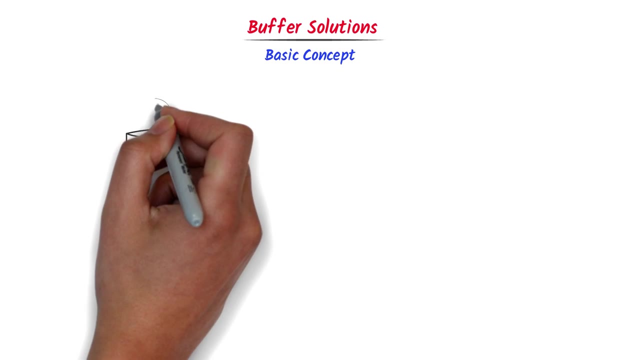 Buffer solutions. Firstly, let me quickly teach you the basic concept of buffer solution. For example, consider water in this beaker. Now I add few drops of acid to this water. We can see that the color of the water changes to red. Thus we say that when color changes, its pH changes. 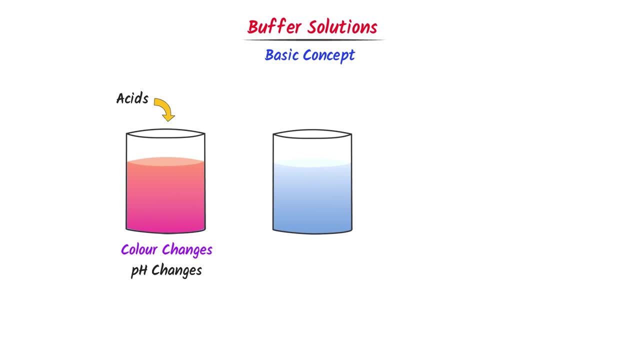 Secondly, consider water in this beaker. Now I add few drops of base to this water. We can see that the color of the water changes to blue. So we say that when color changes its pH changes. Thirdly, consider unknown solution in this beaker. Now I add few drops of acid to this. 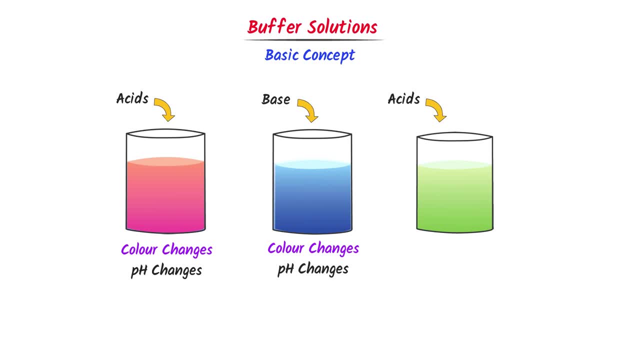 solution. We can see that color doesn't change. Thus we say that no color change means no pH change. Secondly, I add few drops of base to this solution. Again, we can see that color doesn't change. Thus we say that no color change means no pH change. 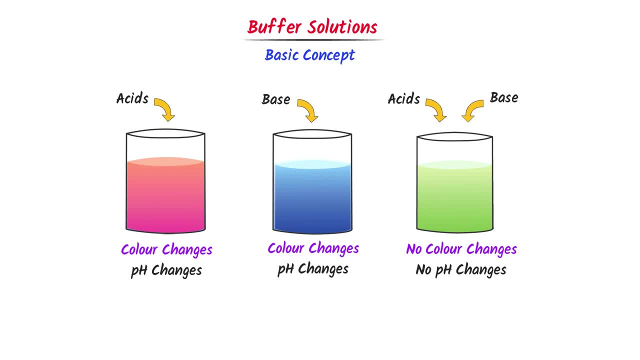 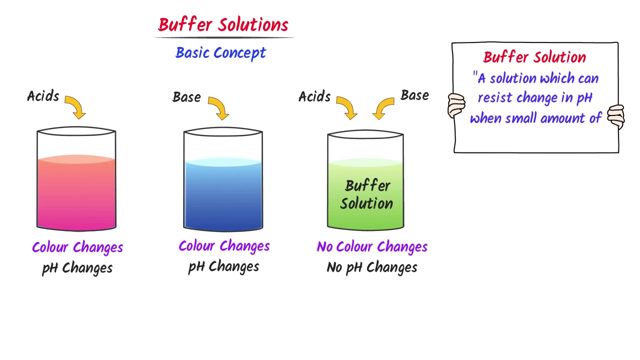 Therefore we conclude that acid and base cannot change the pH of this solution. Thus we say that this solution is a buffer solution. Therefore, we define buffer solution as a solution which resists change in pH when a small amount of acid or base is. 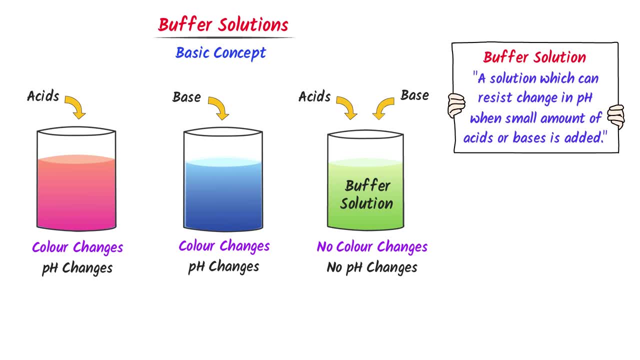 added to it. Let me repeat it: A solution which resists change in pH when a small amount of acid or base is added to it. Note it down that the word buffer means to digest shock. So buffer solution digest the shock of pH. Now let me teach you that. how can we prepare buffer solution? Well, 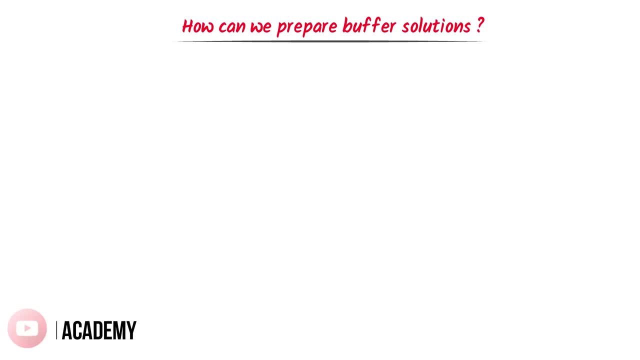 in chemistry there are two types of buffer solutions: Acetic buffer solution and base buffer solution. Remember that here I will teach you my personal method, which some people may do not like it, but it is the most simple one which student easily understand. Now, in case of acetic, 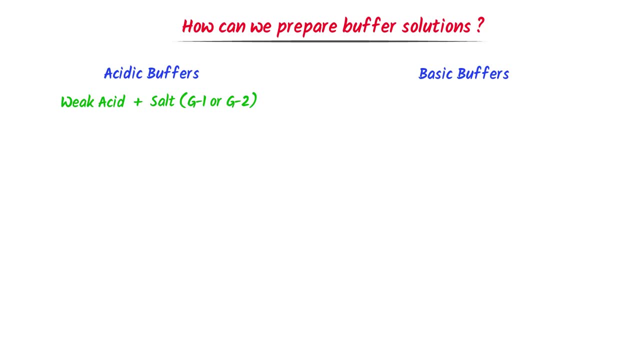 buffer. I will take weak acid plus its salt, with group 1 or group 2 elements. For example, consider hydrogen cyanide. We know that hydrogen cyanide is a weak acid acid. Now I remove hydrogen atom from it and instead of hydrogen I will replace it by sodium. 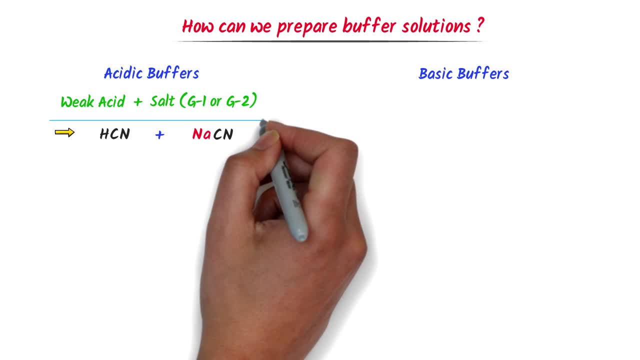 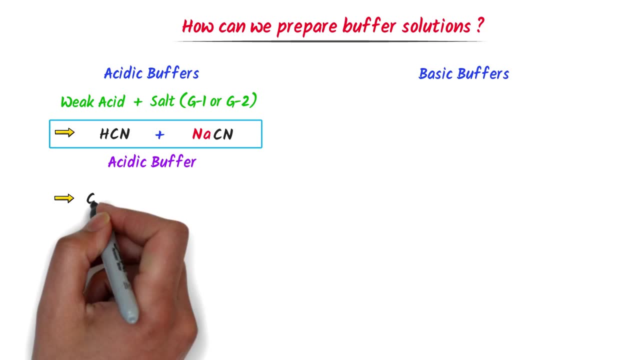 So I get sodium cyanide. Now a mixture of hydrogen cyanide plus sodium cyanide will make acetic buffer solution. Secondly, consider acetic acid. We know that acetic acid is a weak acid. Now I remove hydrogen from it and instead of hydrogen I will replace it by potassium. 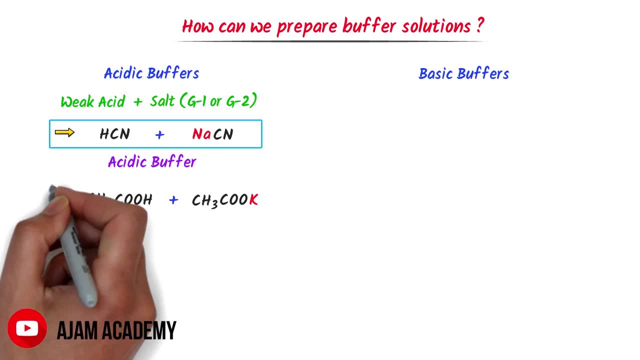 So I get potassium acetate Now, a mixture of acetic acid plus potassium acetate form acetic buffer solution. Thirdly, consider carbonic acid. We know that carbonic acid is a weak acid. Now I remove hydrogen from carbonic acid and instead of hydrogen 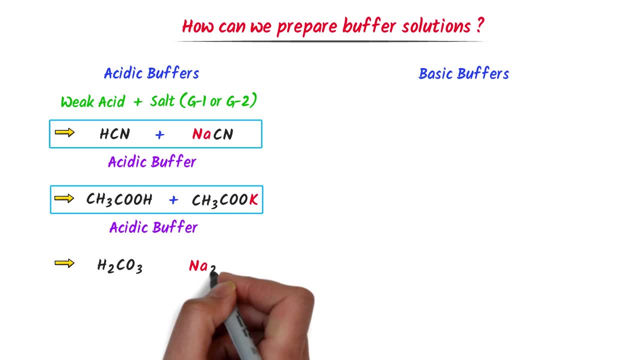 I replace it by sodium, So I get sodium carbonate. Now a mixture of carbonic acid plus sodium carbonate form acetic buffer solution. So by this way we can easily form acetic buffer solution, While in case of basic buffer solution I take weak base and add salt with chlorine. 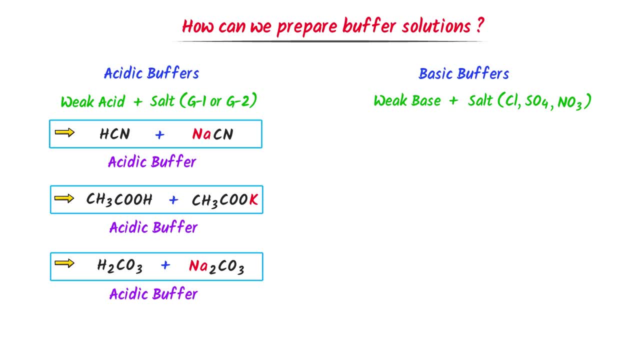 sulfate and nitrate ion, For example. consider ammonium hydroxide. We know that it is a weak base. Now I remove hydroxide ion from it and I replace it by chlorine ion. I get ammonium chloride. Now a mixture of ammonium hydroxide plus ammonium chloride will 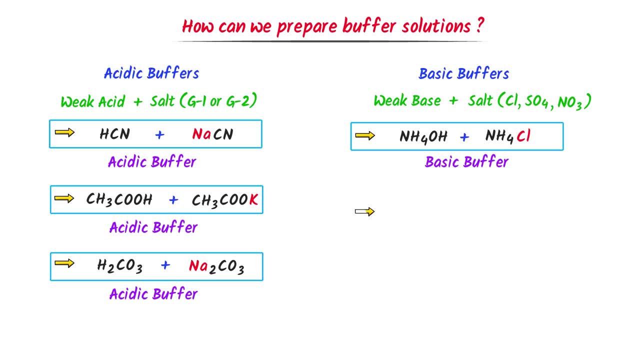 form a basic buffer solution. Secondly, again consider ammonium hydroxide. Now I remove hydroxide ion from it and I replace it by sulfate ion. I get ammonium sulfate. Now a mixture of ammonium hydroxide and ammonium sulfate will form a basic 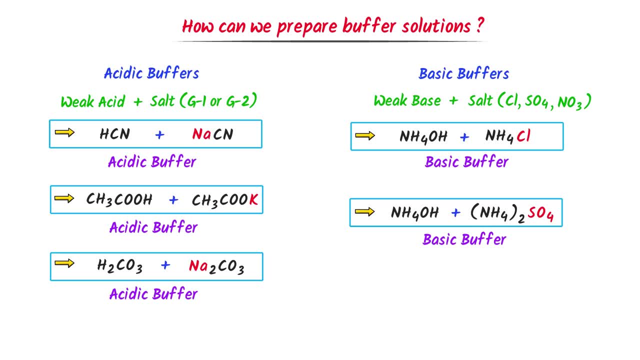 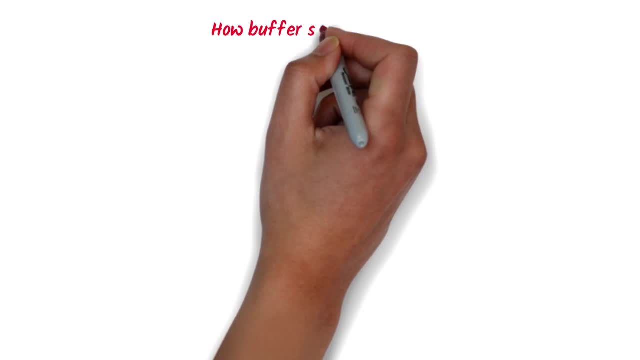 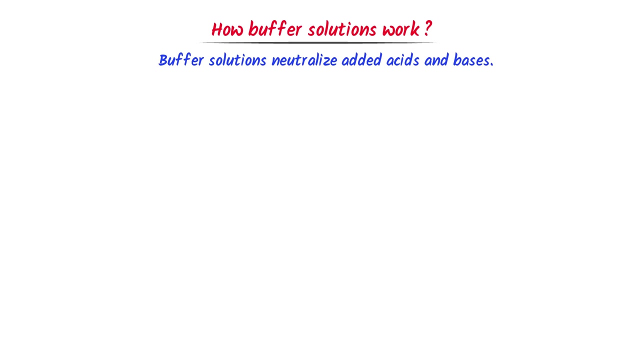 buffer solution. Thus, using this simple method, we can easily prepare acetic buffers and basic buffers. Now let me teach you the working of buffer solution, or how buffer solution maintain constant pH. Well, buffer solution work by neutralizing any added acid or base to maintain the constant pH. Simply remember that buffer solutions maintain the constant. 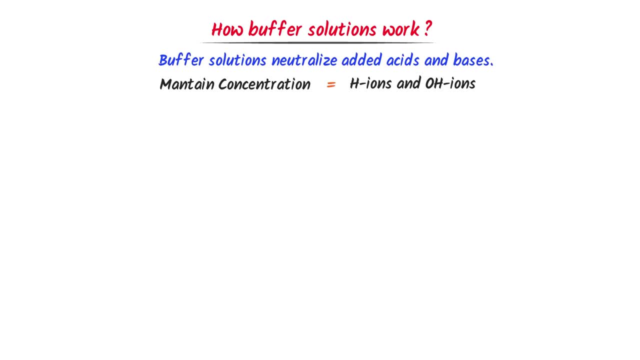 concentration of hydrogen ions and hydroxide ions and add solution. For example, consider acetic buffer solution which contain acetic acid and sodium acetate. We know that acetic acid is a weak acid which partially dissociate into acetate ion plus hydrogen ion. For example, if there are eight acetate molecules it will dissociate into one acetate. 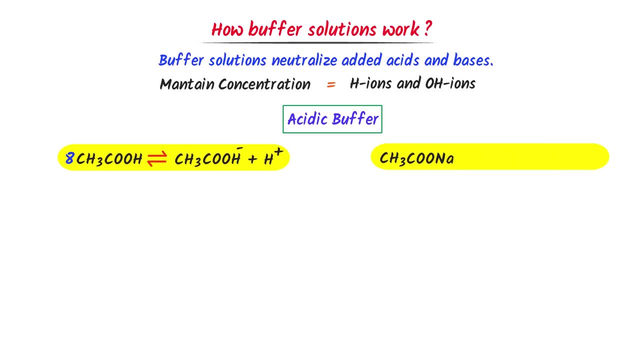 ion and into one hydrogen ion. Secondly, complementary sodium acetate will dissociate into acetate ion plus sodium Ion. Here let's consider that I add potassium hydroxide to this buffer solution. Now this hydrogen ion of the buffer solution will attack on this hydroxide ion. 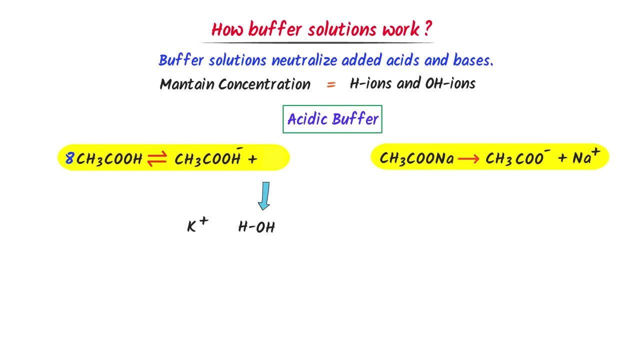 Inieren ion will stop applying vinegar iron to neutralize it by making water molecule, while acetate iron will attack on potassium iron to neutralize it by making potassium acetate. Now, here the equilibrium is disturbed, so acetate iron will dissociate into acetate iron and 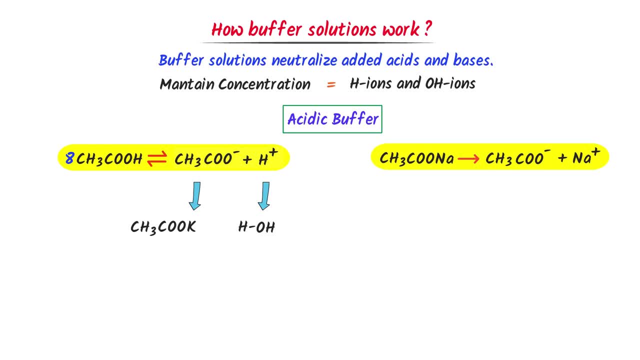 hydrogen iron to maintain the constant pH of the solution. Secondly, consider that I add acid like HCl to this buffer solution. Now this sodium iron of the buffer will attack on chlorine iron to neutralize it by making sodium chloride, while this acetate iron will attack on hydrogen iron to neutralize it by. 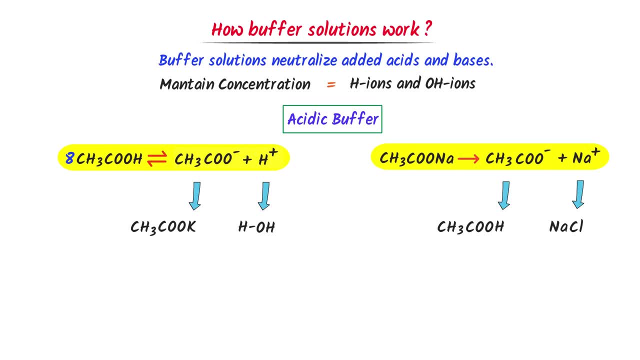 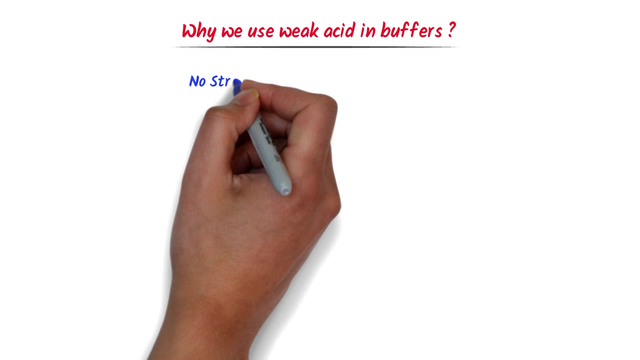 making acetic acid. Thus, by this way, the buffer solution maintained its constant pH when a small amount of acid or base is added to it. it Here. let me teach you one of my favorite questions, which a lot of students do not know to answer: Why we use weak acid and buffer solution. Firstly, remember that we do not use